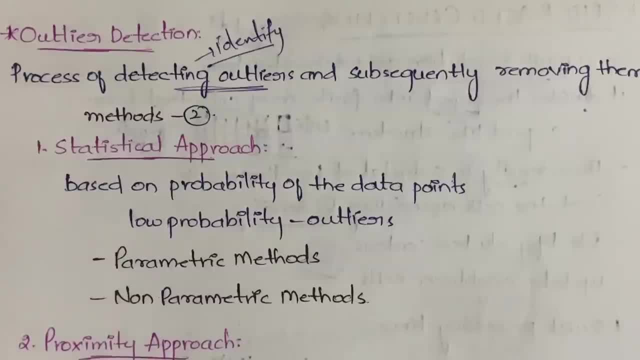 you will be removing them as well. okay, so outlier detection does not only means identification of the outliers, you'll be even removing them as well. okay, just for keeping track. then here you need to work out your data visualization is what we should keep keeping track from. understand this process and then 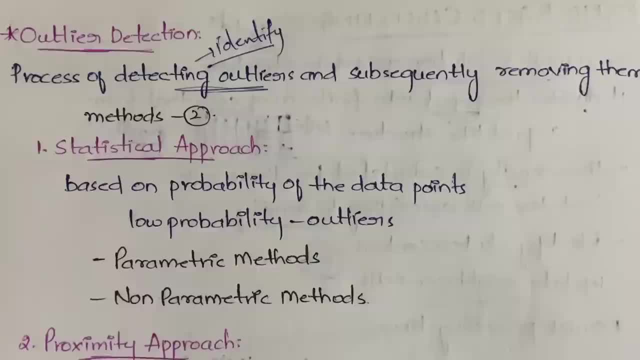 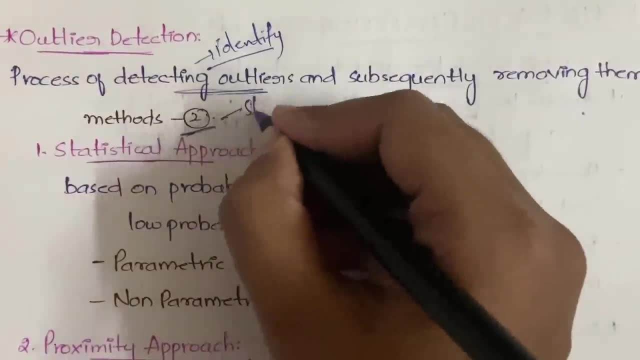 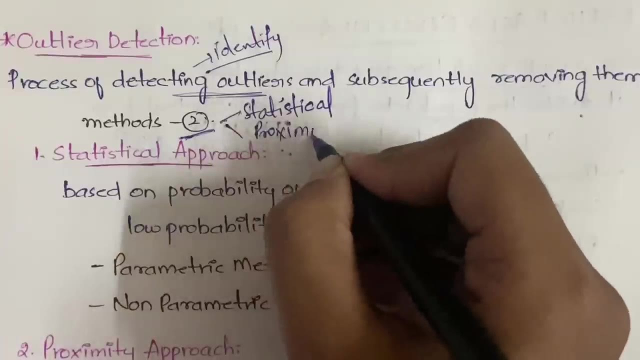 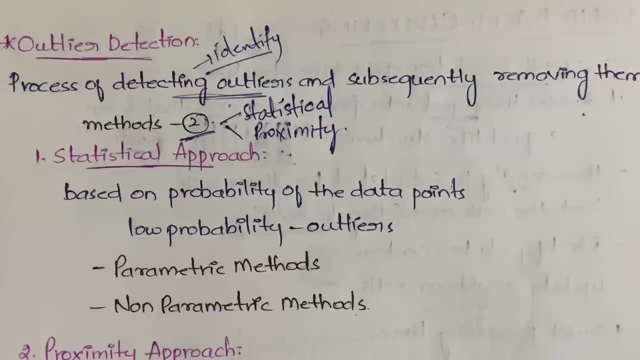 then you can proceed moving on. This is called testing staff, removing them. and in order to do the outlier detection, we have two methods: statistical and the proximity. okay, we have two methods, one statistical and number two is proximity. okay, so what do you mean by statistical approach? is it is based on the probability of the data? 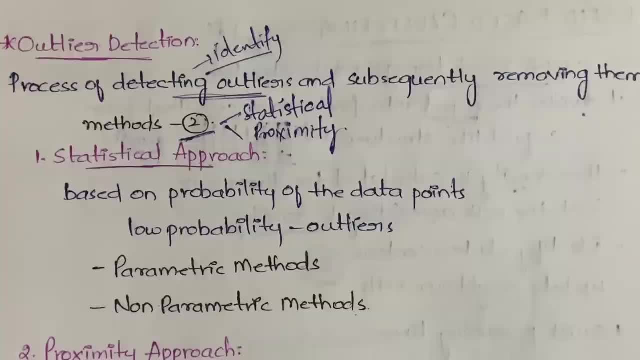 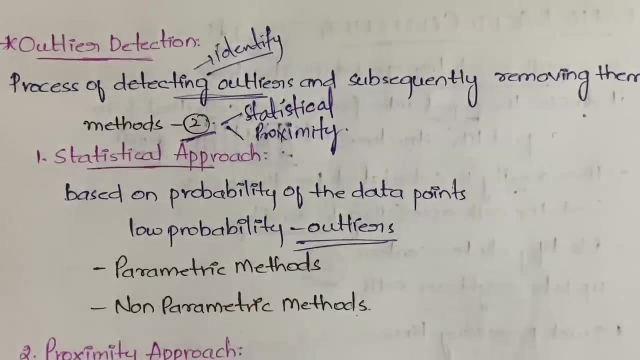 points. suppose you are having 10 data points, then for all those 10 data points you will be calculating the probability. okay, so whichever data point is having the lowest probability, that will be considered as the outlier. so the low probability ones will be considered as the outliers got it. the status statistical approach is basically: it basically depends on the probability. 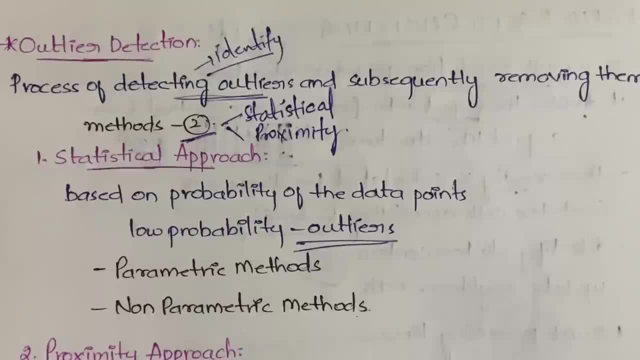 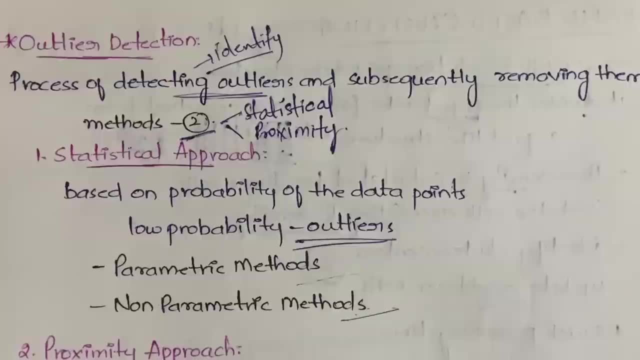 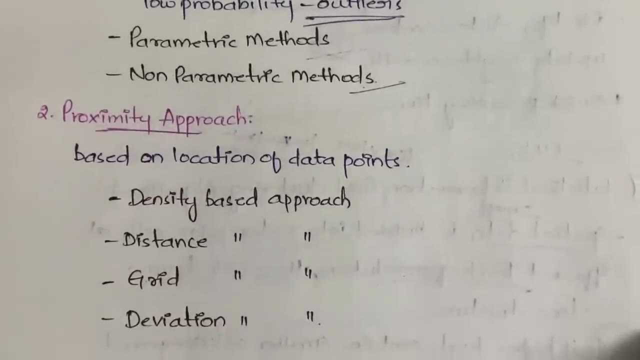 if low probability, you will be categorizing it as a outlier. in this also, we have again two methods: parametric methods and non-parametric methods. i'm not explaining in depth about what parametric and non-parametric in this video. we will be making separate videos for those, okay. next comes a proximity based approach. so in proximity based 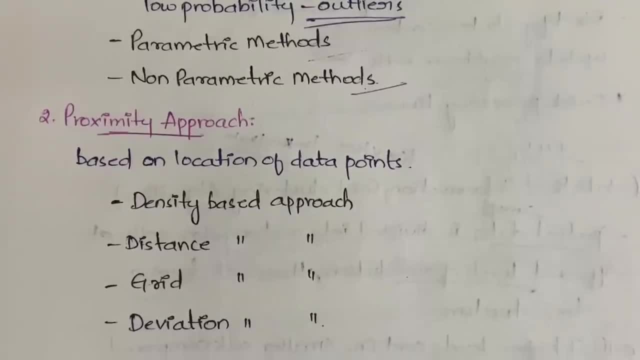 approach. it is based on the location of the data points. location of the data points in the sense: suppose this is our, you know, this is the place where the our data point is supposed to be. suppose you are having all the data points here, like this, like this, like this, and you have one data point away. so, like it depends on the 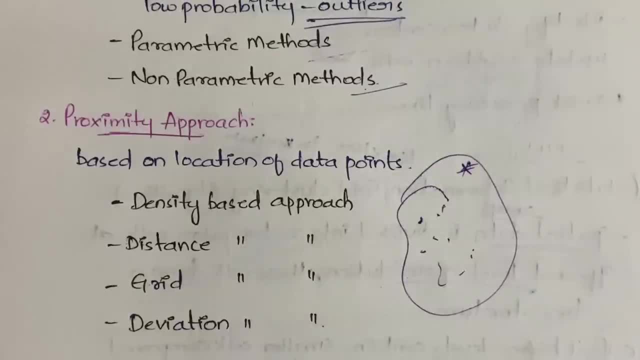 location, whether it is within the cluster or it is outside the cluster, or in the grid or so it. it completely depends on the location of the data point- okay. in this also we again have different types. first is density based approach- okay. second is distance based approach- okay. third is grid. 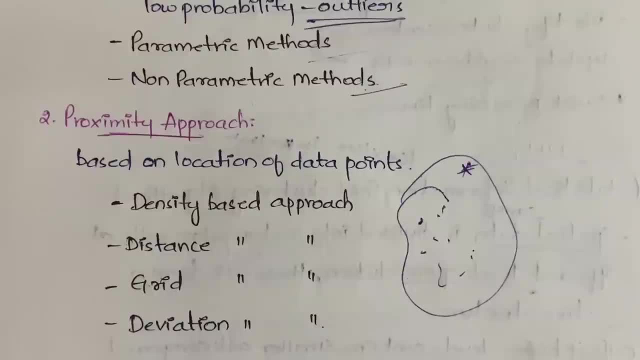 based approach and fourth is deviation based approach. so about all these also separate, separate i'll make. so this is all about the outlier detection methods, two methods, and then those two also statistical proximity. in those two also we have more sub methods. okay, now next types of outliers. so in types of outliers we actually have three types. they are very easy. 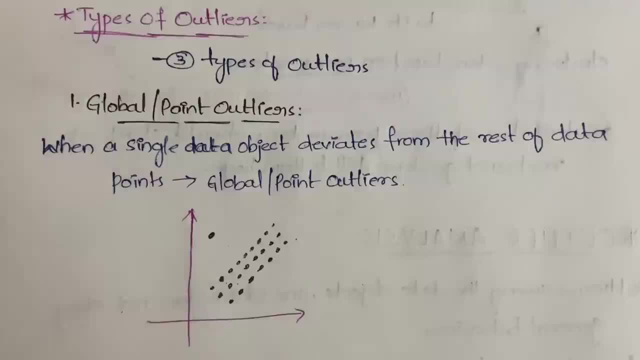 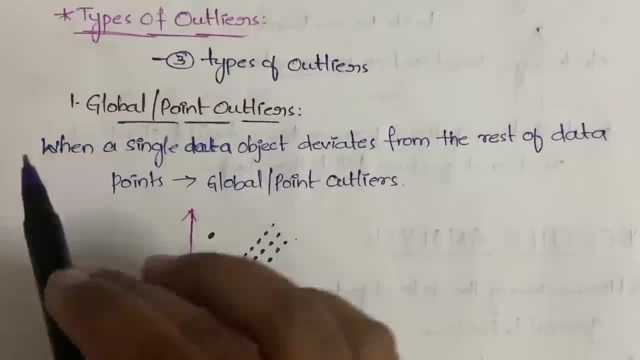 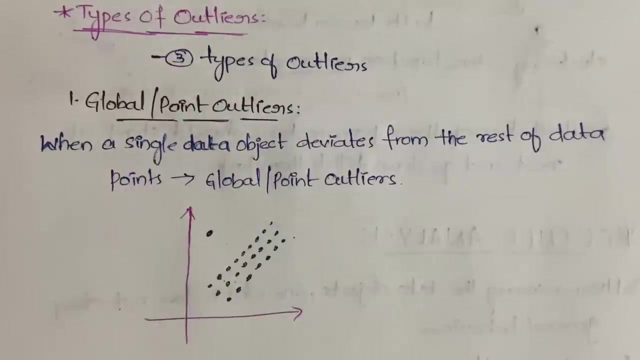 first one is the global or point outliers. second one is the collective outlier. third one is the contextual or conditional outlier. so first is global. global means nothing, but when a single data deviates from the rest of the data points, the such outliers are called as the global or point. 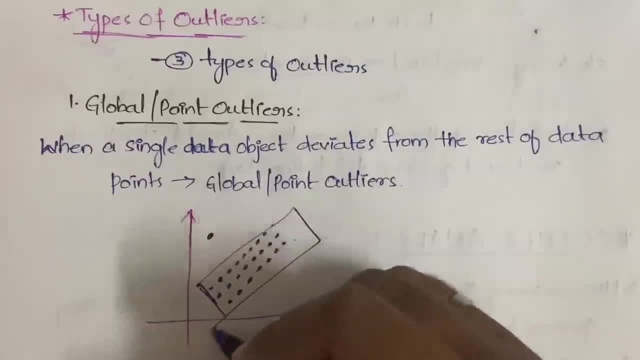 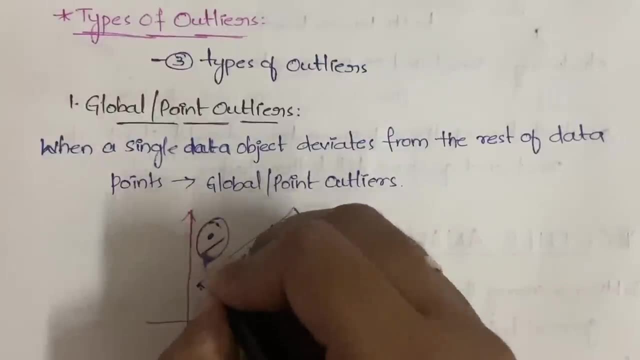 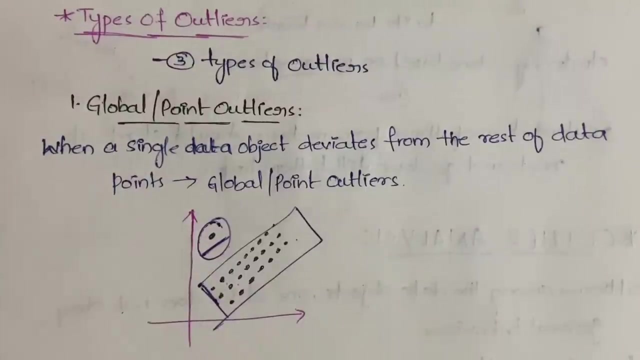 outliers. see, here we have all the outliers in this way, right here we have every, all the outliers that one place in a particular order. but this, the single data object, sorry data objects. this single data object is not in general behavior with them, it is not alone with them, right? they forced them. 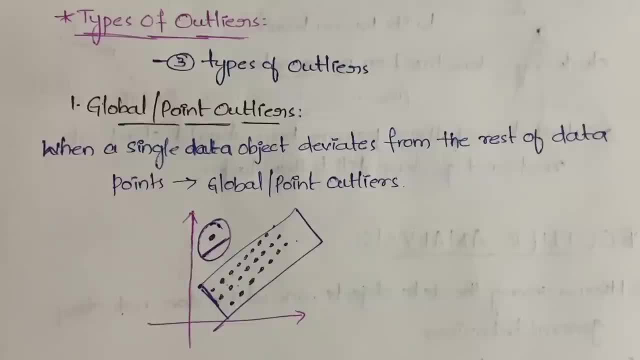 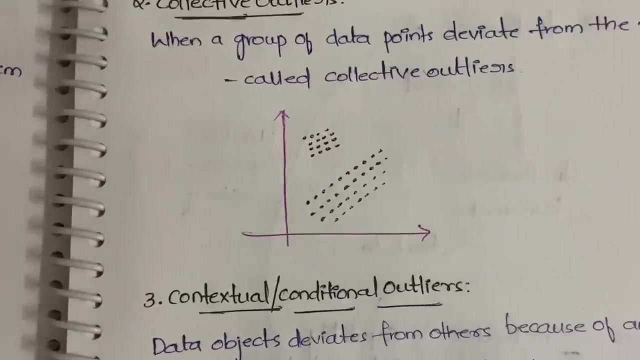 so it is not obeying the general, its behavior. that is, only single data point will not obey, not a group of data points got it only. if single, one or two data points are not obeying, they will come under global or point clusters. next collective clusters. so collective clusters are nothing but in the global or point what we 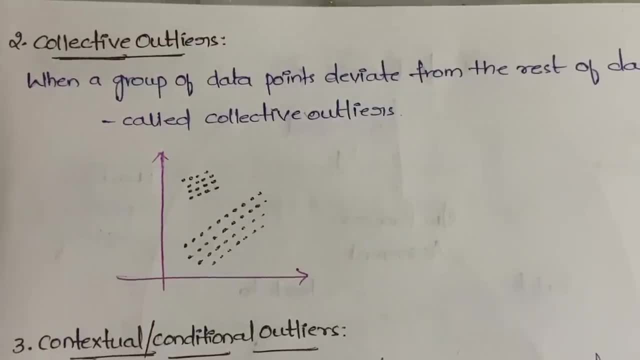 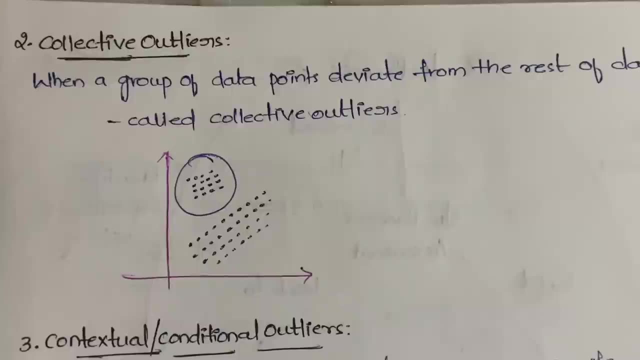 have. we have single data point is not obeying right. but here we will have the group of data points. group of data points will deviate from the actual behavior. it is called as the collective. the word collective itself says right. so the group of data points will be deviating away. okay, done. 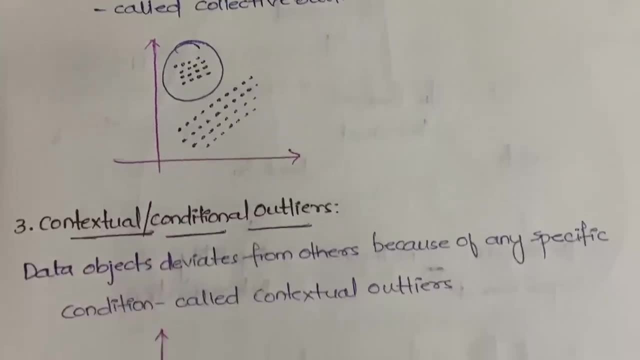 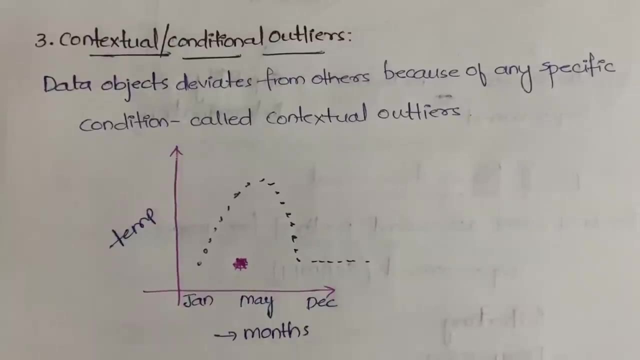 next, after collective, we have the last type, that is the contextual or conditional outliers. so contextual or conditional outliers is nothing but data objects will deviate from others because of any specific condition. so it could be any specific condition. then it is called as the contextual outliers suppose. in january usually the temperatures will be very minimum right, so gradually by the time of may it will reach to the maximum and from may again it will start decreasing till december. so if at all suddenly in may, if the temperature drops to the temperature that we see in january, that is it drops to 10 degrees or 15 degrees celsius, then because of some condition something has happened. 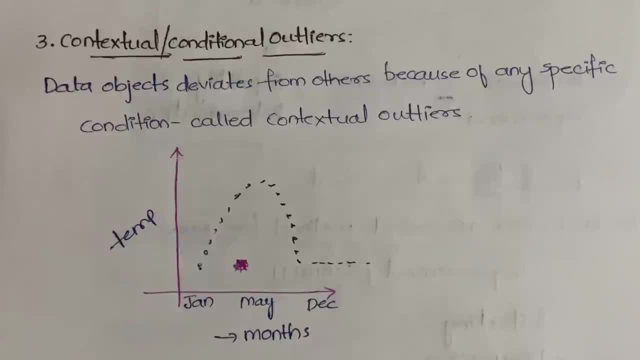 like you know, a flood or some, some because of something, because of some unconditional reasons, the temperature has dropped right. so because of any specific condition, it is not obeying the general behavior. then it is called as the contextual, based on particular context or based on particular condition it is not obeying.